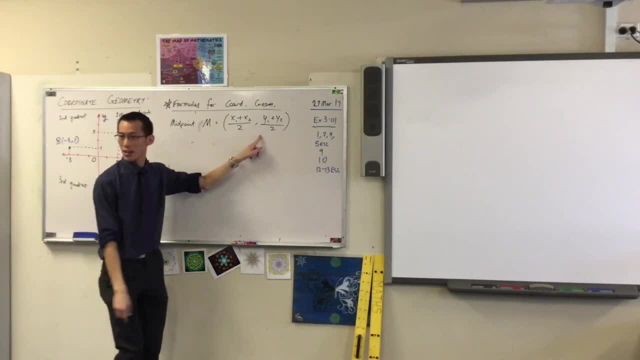 You've got your brackets around the edges, you've got a comma in the middle. there's an x coordinate and a y coordinate For each one. you're adding points, You're dividing them and then you're dividing by two. All you're doing is you're working out the average. 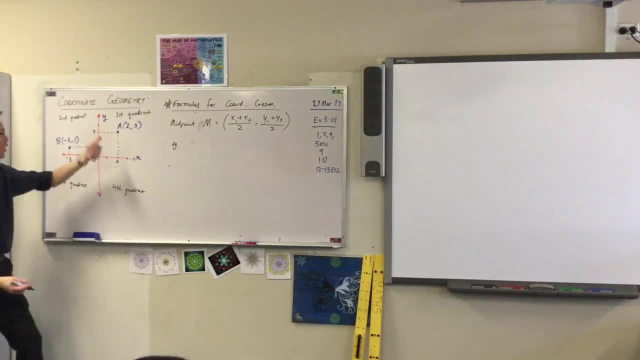 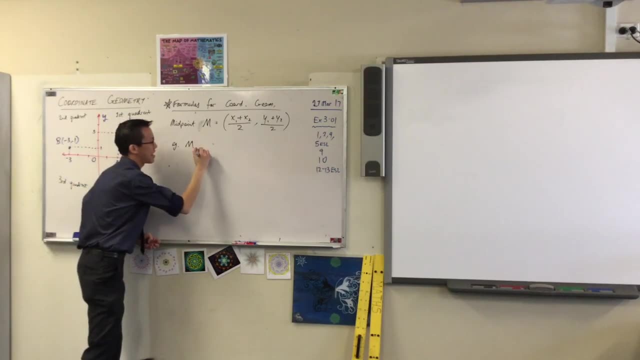 That's all you're doing. So, for example, let's say the midpoint of these two guys over here, So I'll write that as midpoint, and because it's between A and B, I'll write A, B down here, And then I'm going to look and I'm going to say 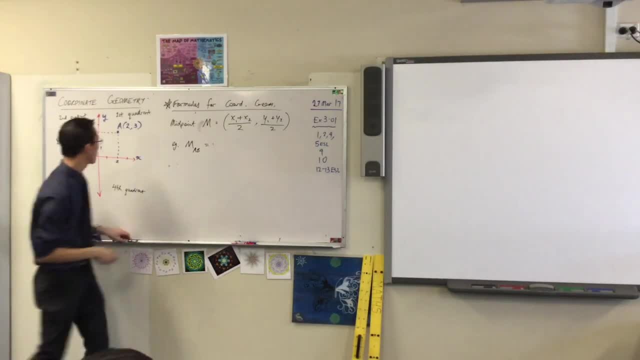 okay, which of these are my x coordinates and which ones are y's. Now, if you've got another colour there, I'm going to go to orange, If you've got another colour there, this is really useful. I'm actually going to label onto my coordinates. 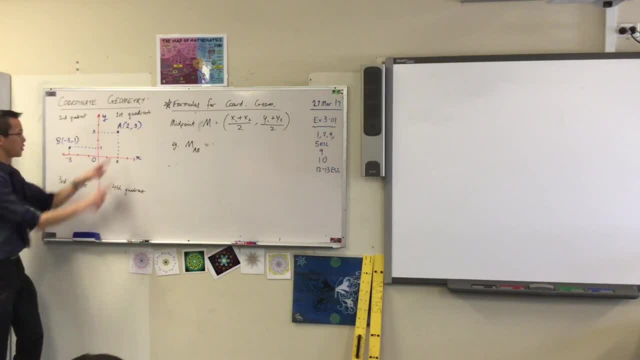 which ones are the x's and which ones are the y's. So have a look here. Two comma three, Which one's the x and which one's the y. again, Two is x, The x is the two, Yeah, And the three is the y. 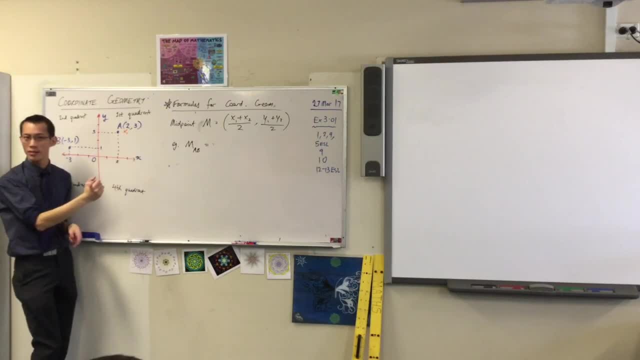 It's alphabetical, Do you remember that? So I'm going to write this as x one, y one. You don't have to do this, but I highly encourage you do, because then you can have it in front of you. Oh, this is which one? 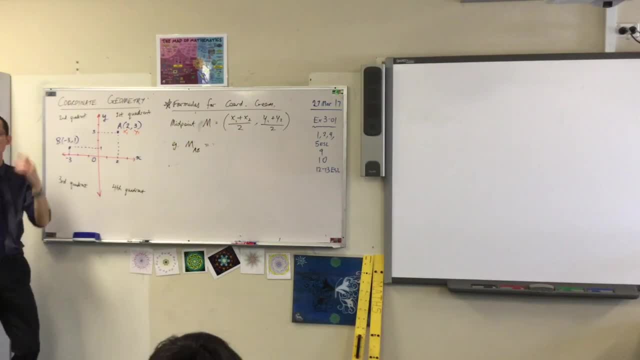 Which number fits where, Rather than trying to keep it all in your head and then mixing them all by accident. So you've got one point and it's x and y, And then you've got the other point, And it also has an x and a y. 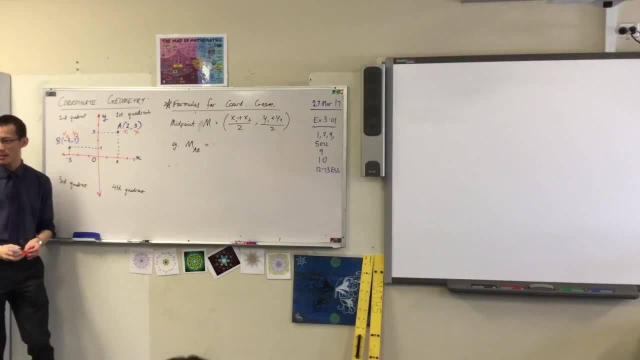 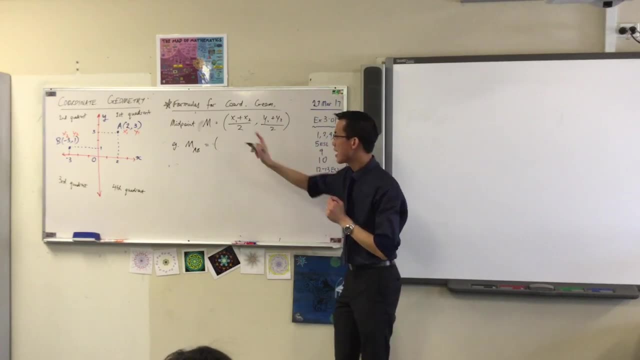 x two, y two. Does that make sense? Right? Let's crunch it and see what happens. So we'll do the x's first, x one plus x two, There's two and there's negative three. So two plus negative three. 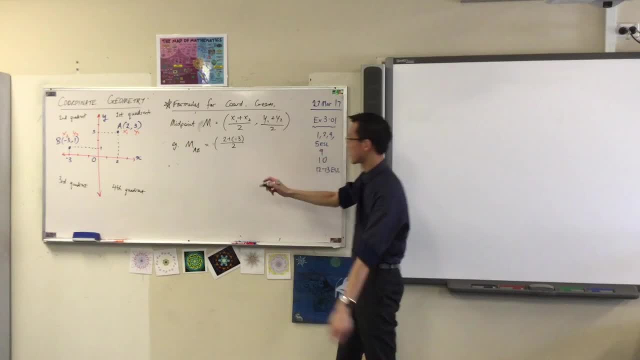 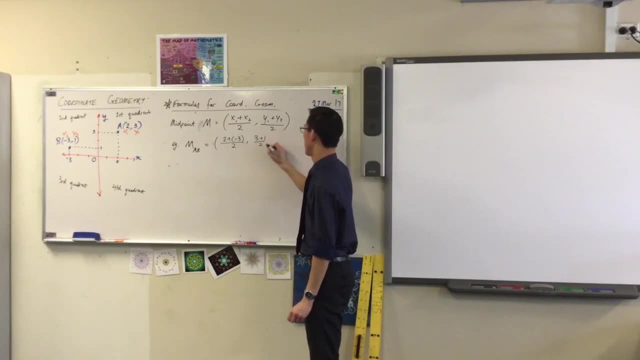 And then I divide by two. There's the x's. What am I going to put in for the y's? Three plus one Over two. Okay, I'm just going to quickly calculate this. I could go to my calculator, but these are pretty simple numbers that we started with. 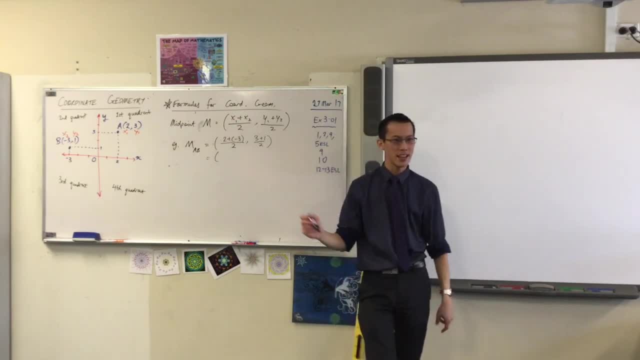 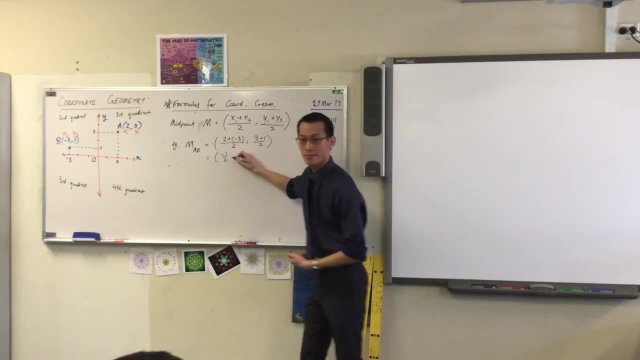 So two plus negative three is two minus three, Yes, Which is negative one. So this is just negative one over two. What about on the right hand side? What am I getting here? Four over two, Four over two, which is. 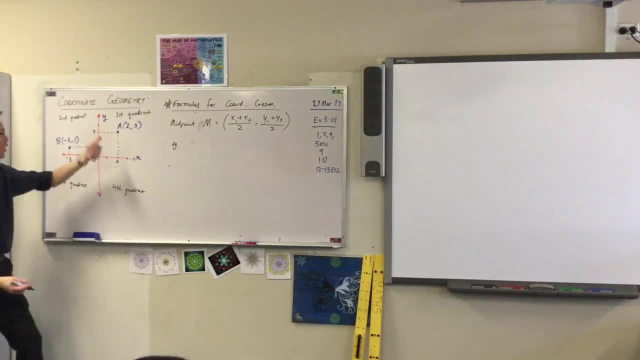 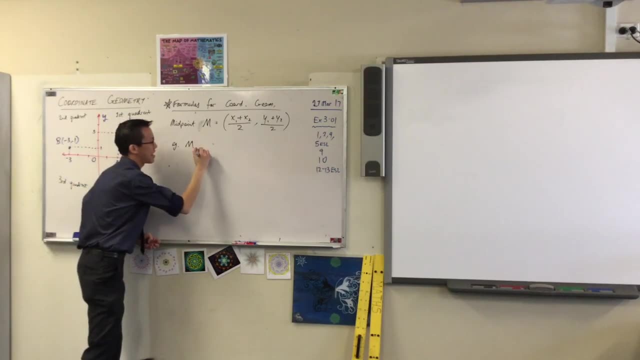 That's all you're doing. So, for example, let's say the midpoint of these two guys over here, So I'll write that as midpoint, and because it's between A and B, I'll write A, B down here, And then I'm going to look and I'm going to say 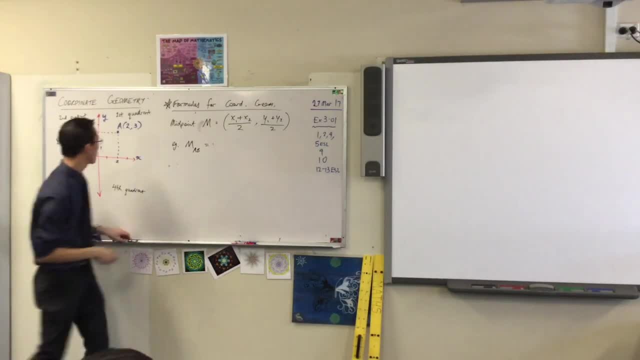 okay, which of these are my x coordinates and which ones are y's. Now, if you've got another colour there, I'm going to go to orange, If you've got another colour there, this is really useful. I'm actually going to label onto my coordinates. 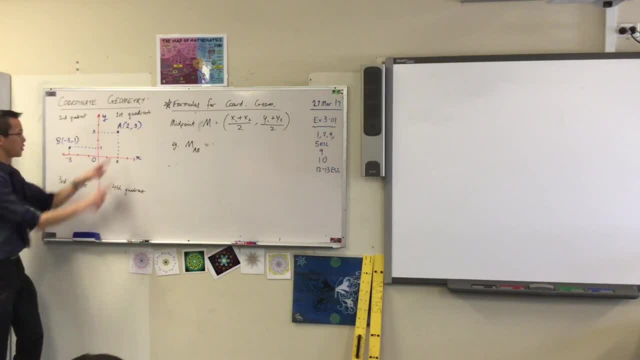 which ones are the x's and which ones are the y's. So have a look here. Two comma three, Which one's the x and which one's the y. again, Two is x, The x is the two, Yeah, And the three is the y. 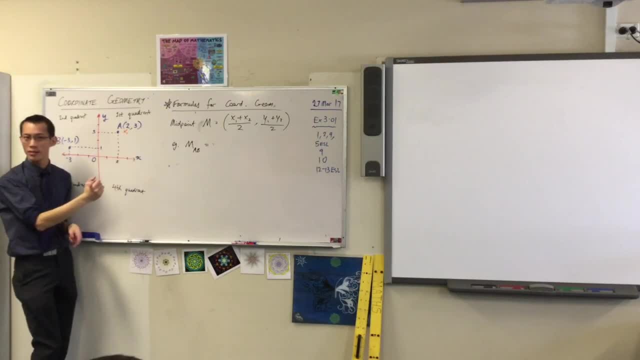 It's alphabetical, Do you remember that? So I'm going to write this as x one, y one. You don't have to do this, but I highly encourage you do, because then you can have it in front of you. Oh, this is which one? 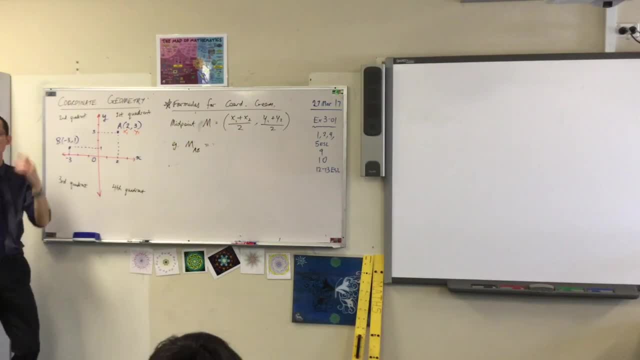 Which number fits where, Rather than trying to keep it all in your head and then mixing them all by accident. So you've got one point and it's x and y, And then you've got the other point, And it also has an x and a y. 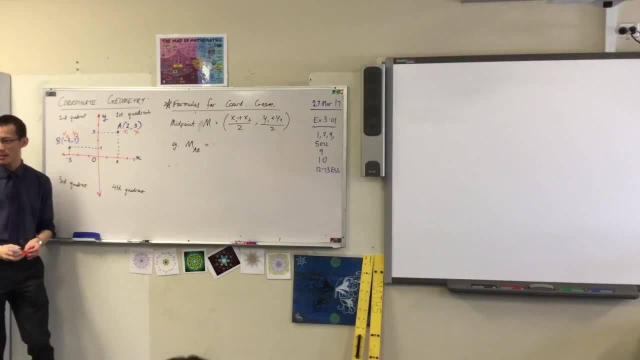 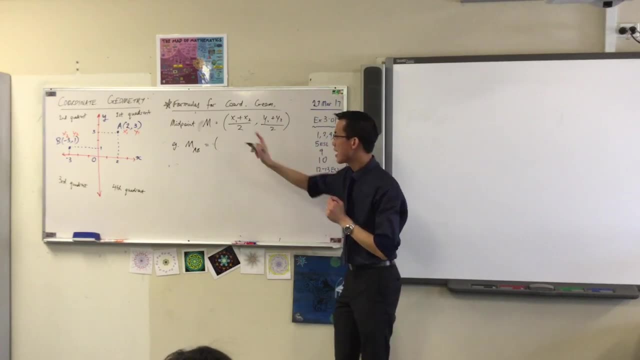 x two, y two. Does that make sense? Right? Let's crunch it and see what happens. So we'll do the x's first, x one plus x two, There's two and there's negative three. So two plus negative three. 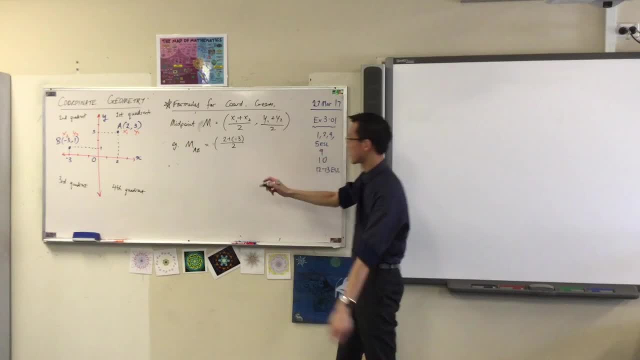 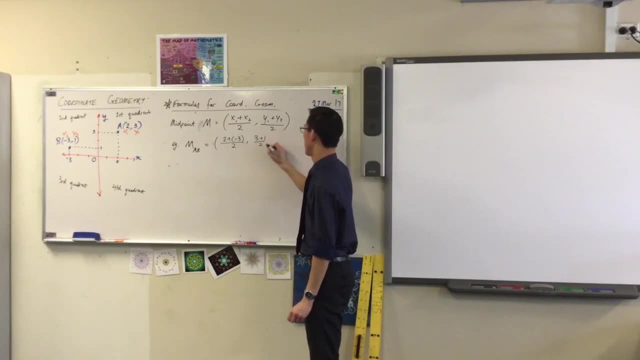 And then I divide by two. There's the x's. What am I going to put in for the y's? Three plus one Over two. Okay, I'm just going to quickly calculate this. I could go to my calculator, but these are pretty simple numbers that we started with. 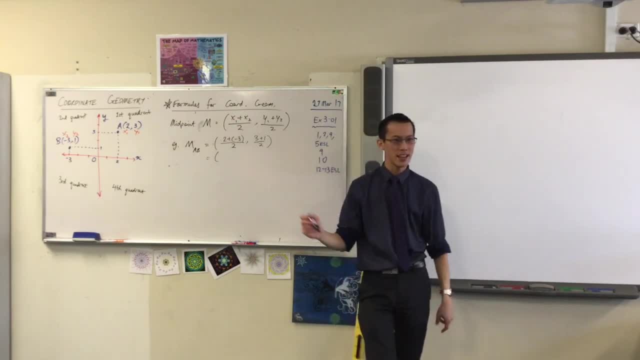 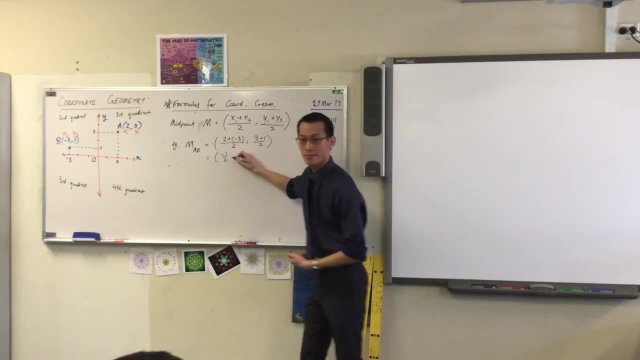 So two plus negative three is two minus three, Yes, Which is negative one. So this is just negative one over two. What about on the right hand side? What am I getting here? Four over two, Four over two, which is. 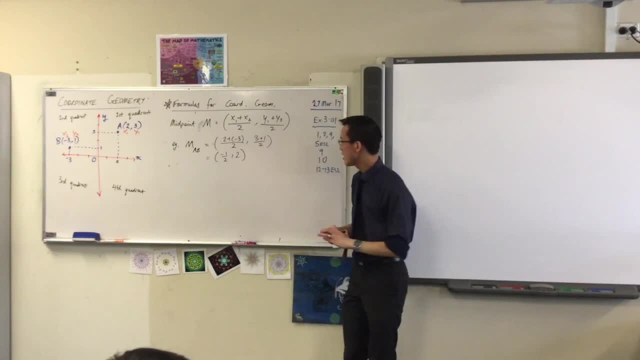 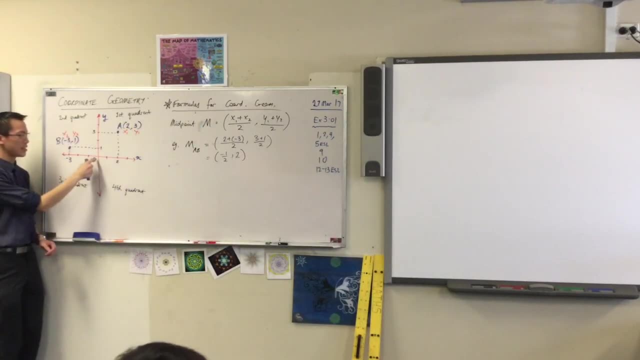 Two, Two. Okay, Now you can see. I can actually find where this is on my original diagram. Let's go and have a look. Negative a half, Here's zero, and here's negative one, Do you agree? So negative half is halfway in between here and here.